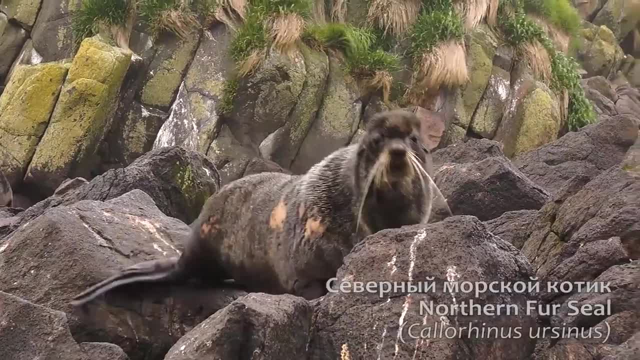 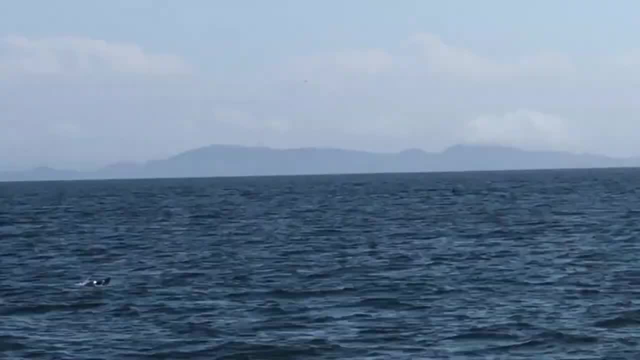 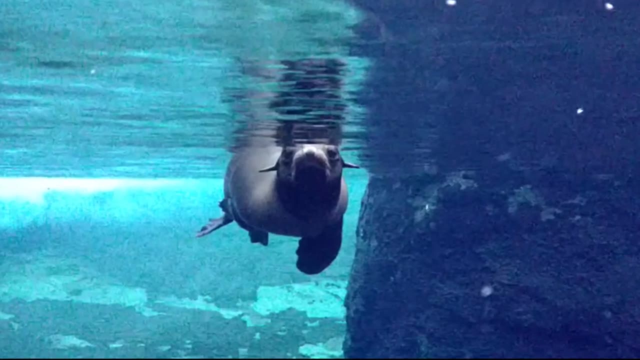 They have whiskers on their snout. Their fore flippers are very strong so that they can walk or run on all fours or climb steep cliffs. They spend most of the year more than 300 days in the ocean. They are thought to be mostly solitary at sea. They primarily use 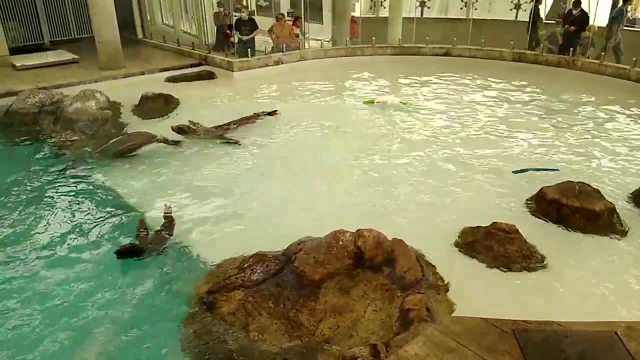 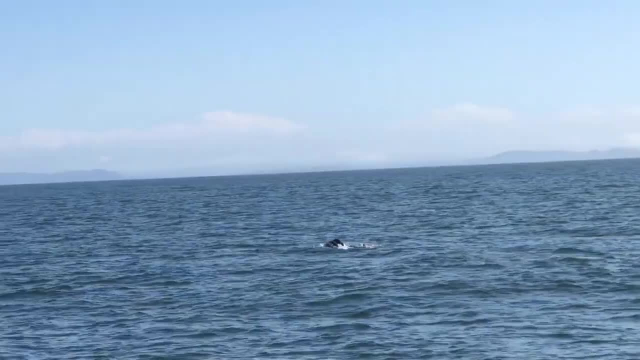 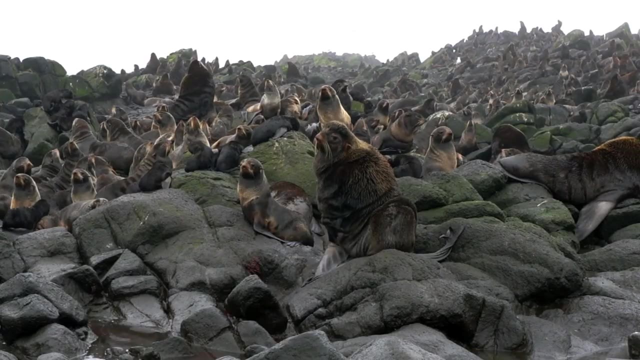 the open ocean for foraging and rocky beaches for reproduction. Northern fur seals eat a wide variety of squid and schooling fish. They mainly feed at night, when prey species are closer to the ocean surface. Males are significantly larger than females. Males can grow to 7 feet long and weigh up. 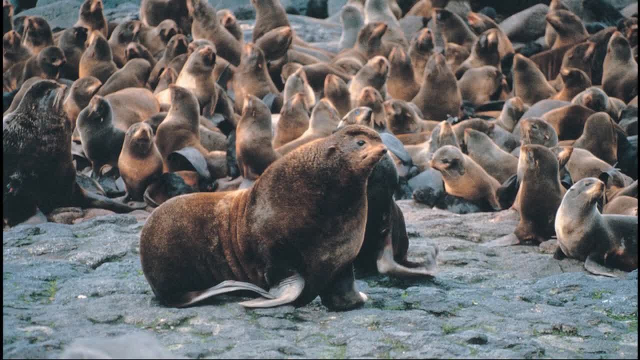 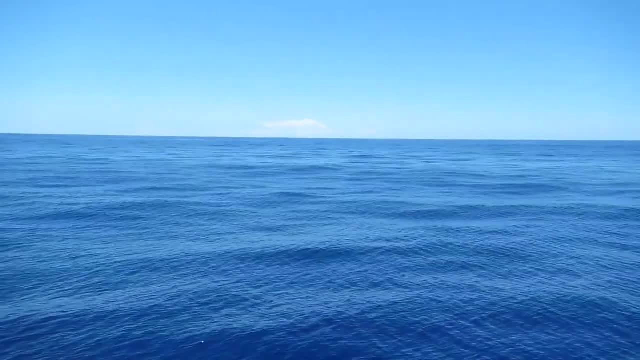 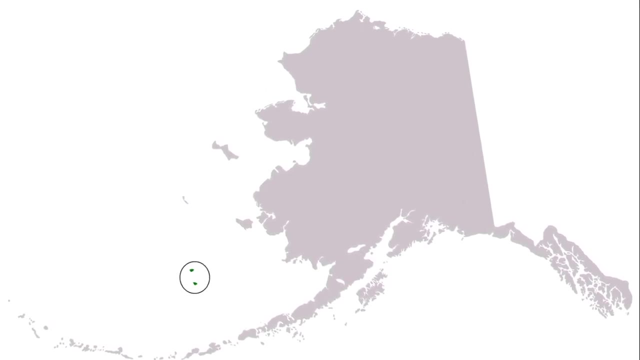 to 600 pounds, while females can only grow to 5 feet and weigh up to 120 pounds. In the spring, most northern fur seals migrate north to breeding colonies in the Bering Sea. Alaska's Pribilof Islands are the breeding grounds for more than two-thirds of the world population. 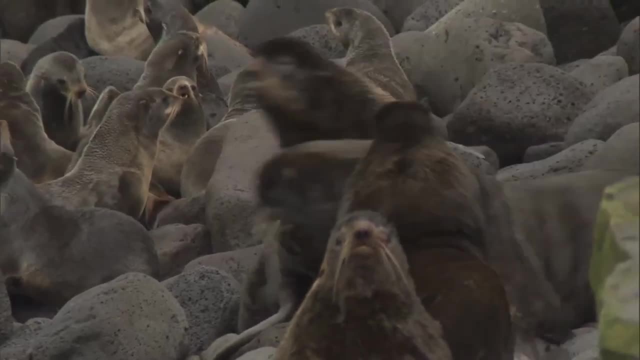 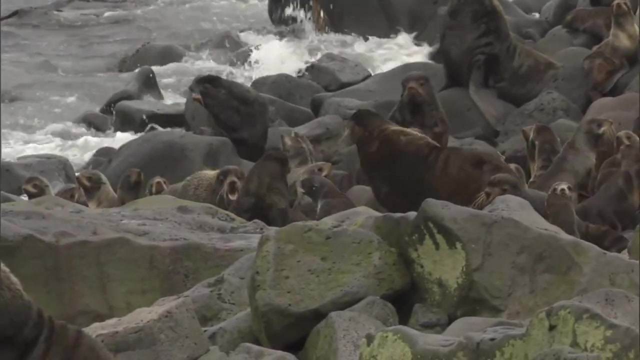 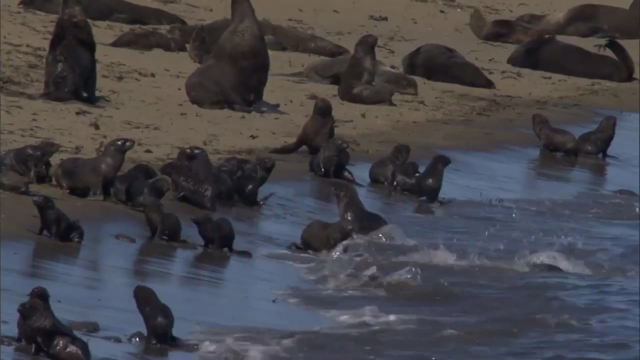 of northern fur seals. Each year, large males called bulls arrive first to establish territories that they will aggressively defend. As many as 100 females may show up within each of these territories. Females generally have their first pup at 5 to 6 years of age and often have an affinity. 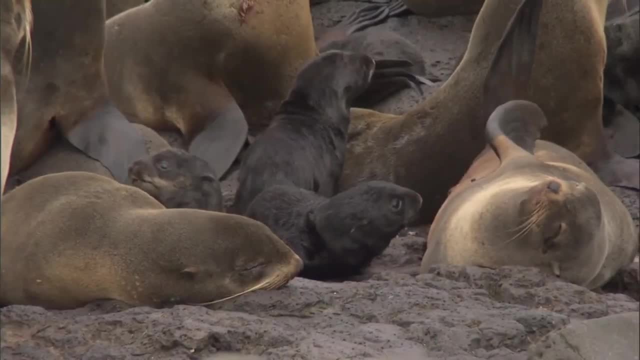 for a specific breeding site. They typically start returning to their breeding sites in late June and give birth to a single pup shortly after arriving at their first breeding site. They usually start returning to their breeding sites in late June and give birth to a single pup shortly after arriving at their first breeding site. 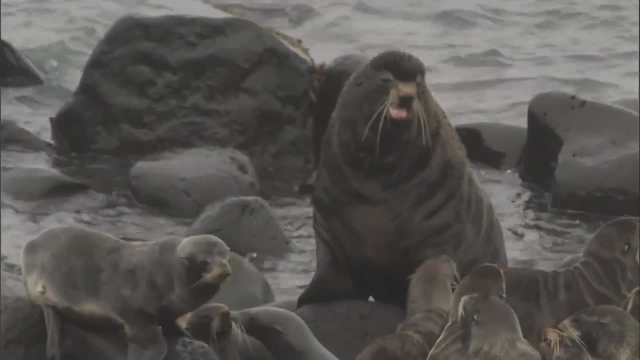 They usually start returning to their breeding sites in late June and give birth to a single pup shortly after arriving at their first breeding site. Then they mate again within a week. Pups are black in color until they molt at around 3 months old and become a silver-gray. 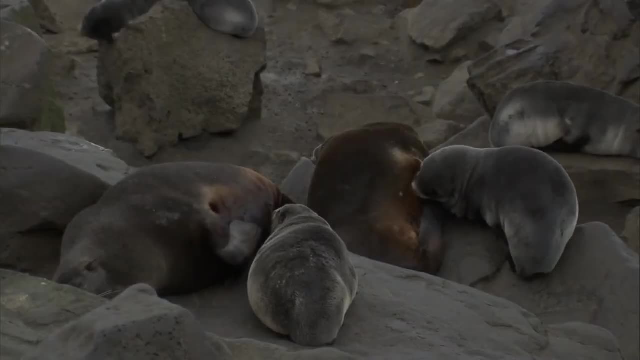 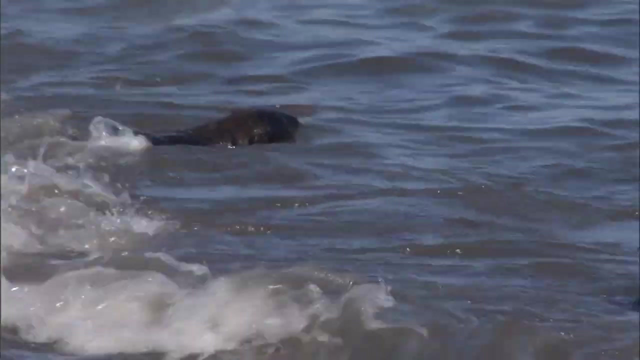 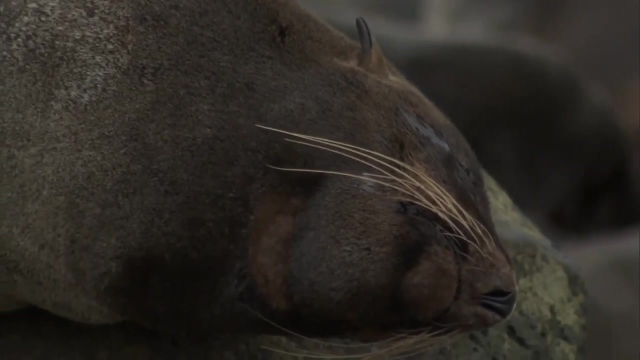 color Females nurse their pups for about 4 months, making several week-long trips to sea to feed during this period. Then the pups leave the breeding site and begin to forage independently. Northern fur seals can live around 26 years. They are preyed on by animals like killifish. 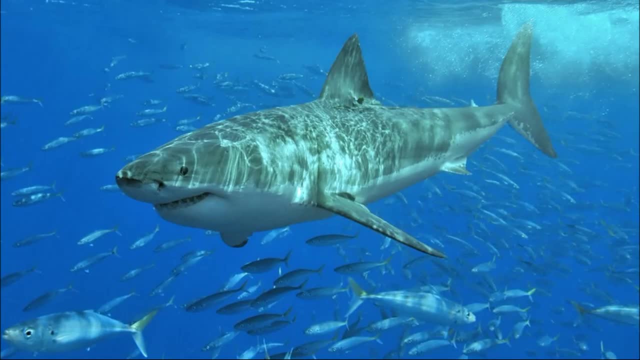 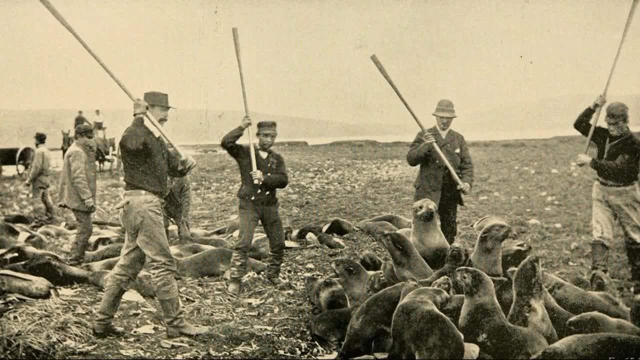